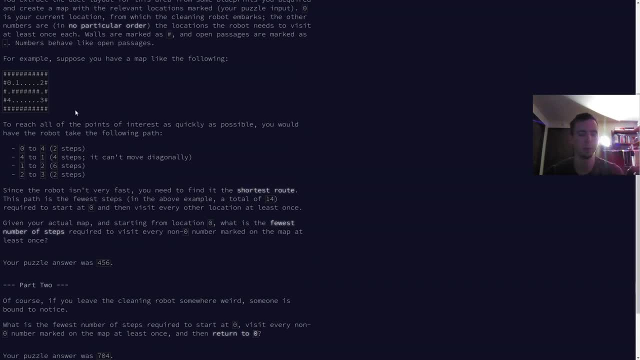 I'm just going to do the breadth-first search and parsing parts of the problem. But I'm going to do it in Haskell today and I'm going to write it in a pure functional way as one does in Haskell, and just I'm kind of doing this mainly to contrast the Python version which you know. 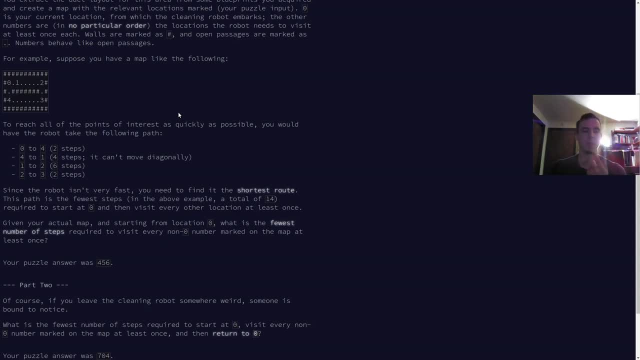 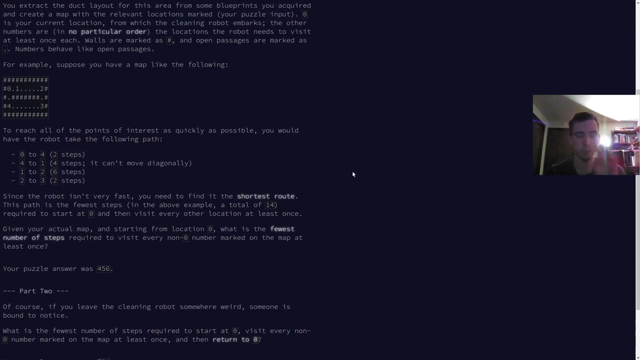 is an imperative style with the Haskell style, and show that in a lot of ways they're really not hideously different and even algorithms like this lend themselves really well, actually, especially algorithms like this lend themselves really well to functional programming patterns and paradigms. So really quickly to reiterate the problem, basically we're given a grid of data. 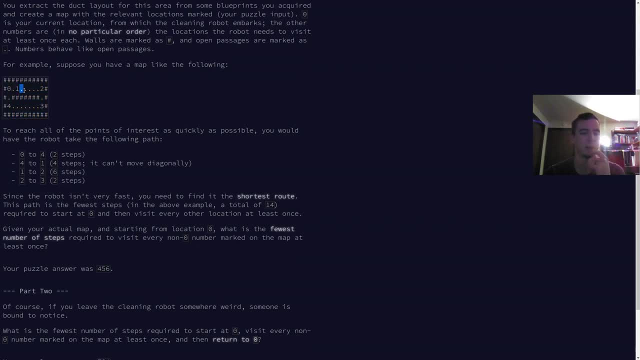 and the grid has these numbers on it, And there's also these dots which indicate paths that we're allowed to take, And there's these hash characters which indicate walls that we're not allowed to step over, And the overall problem wants you to know how, what the shortest path is through all the numbers. 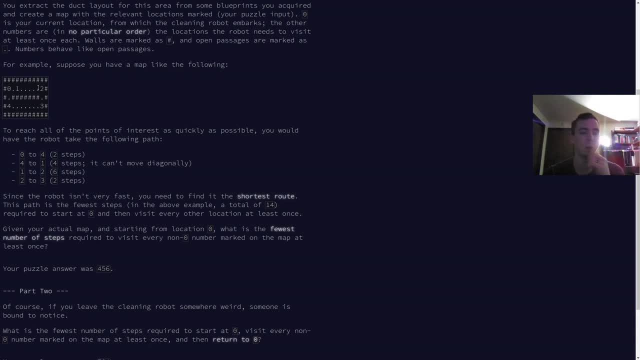 In this case it happens to be 0 to 4,, 4 to 1,, 1 to 2, and then 2 to 3.. But in this problem I'm not going to solve the shortest path problem, I'm not going to solve the overall shortest path problem. 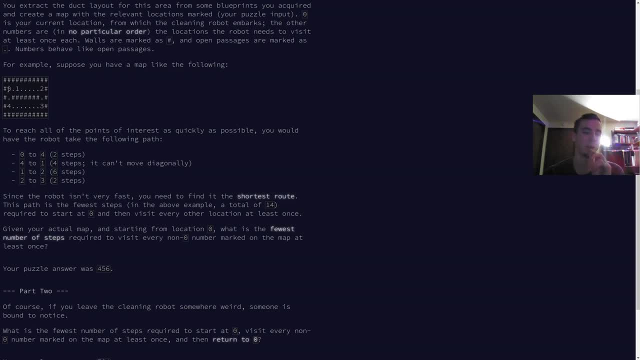 We're just going to solve the small shortest path problem. finding the shortest path, for example, from 0 to 3, or from 0 to 1.. So that's the plan for this video. So if you haven't seen the Python video and you'd like to watch it, go ahead. 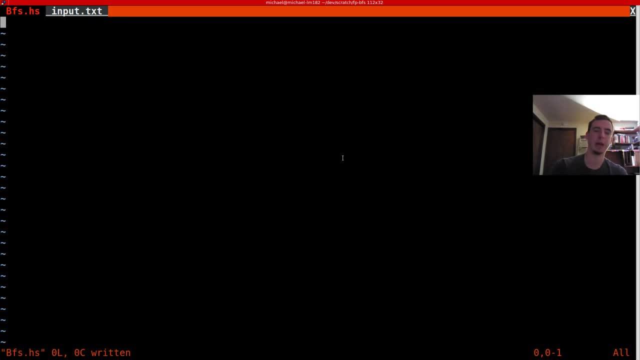 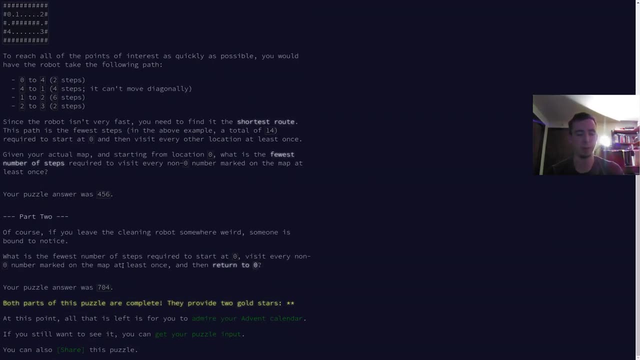 But anyways, we're going to do it in Haskell this time around. So here I have breadthfirstsearchhaskell And here I have a small input. this is the small example. The larger example is much crazier, but we'll just use the small one for now. 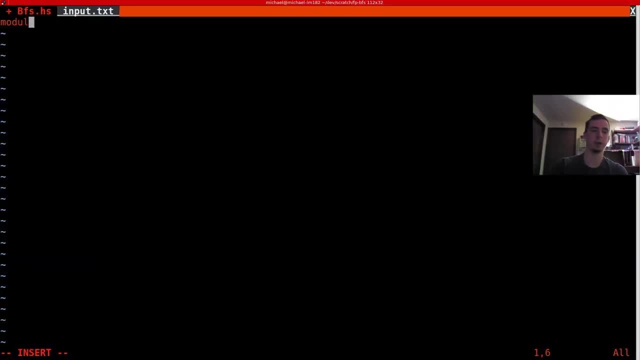 The solution should work for the large one as well. So in Haskell, we start out by saying module main, Which will contain our actual code. Now there are three structures that I'm going to use, three collections types that I'm going to use to actually implement this. 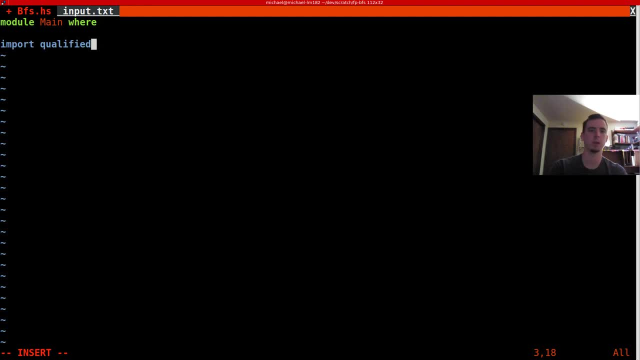 So we're going to import qualified datasequence as seek And I'm going to use a sequence to represent the to try list. Or, in other words, as we're searching, things that we have to try to investigate later are going to be stored in this sequence. 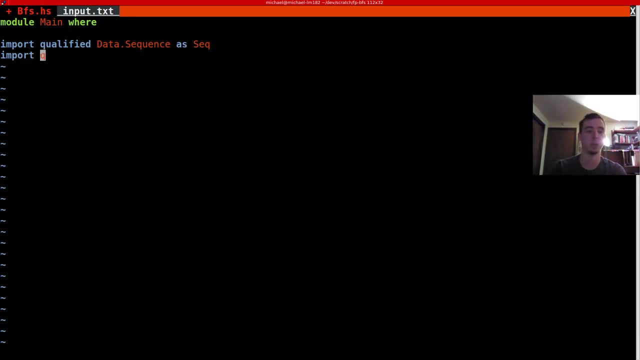 Basically because it makes a nice in-memory queue. So dataset I'm going to import as s And these will get confusing. I'm sorry about that. I don't really know a much better way to structure it. honestly, Datamapstrict as m. 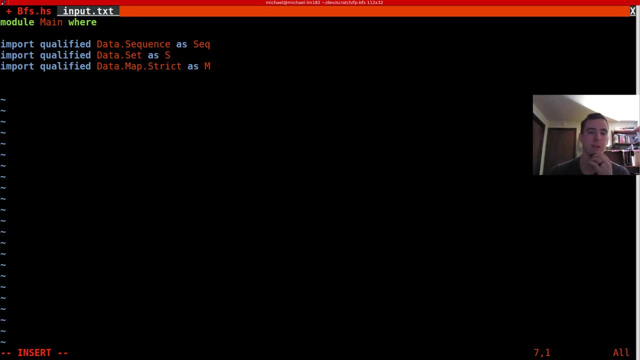 So we're just going to import these things And they're going to be qualified such that we have to reference them by their aliases, Which is the as part. So I'm also going to create a type to represent positions, And positions are just going to be a tuple of x, y coordinates. 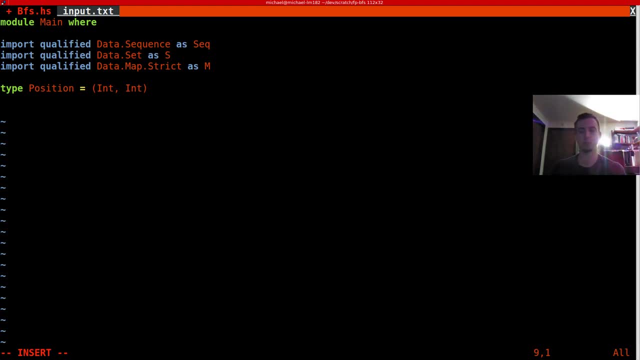 So in the last problem, the way I solved it was, the first thing I did was I parsed out all of the positions which I called spots, And I parsed out a lookup from our numbers in the problem, Because we actually care about these numbers and how to get to other numbers. 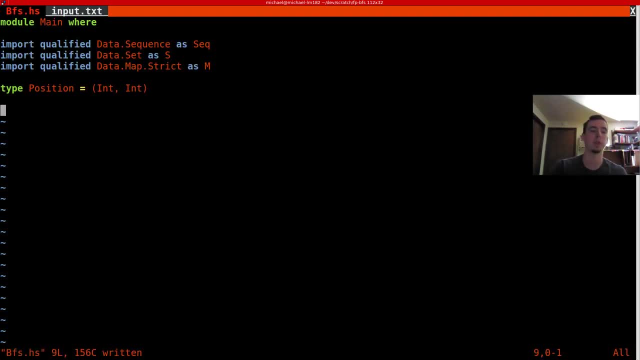 And we're allowed to step over numbers. I parsed those things out. So we're actually going to do a lookup from a number to its position. So we're actually going to do the same thing here. So spots and positions is going to be a function which is going to take in a string. 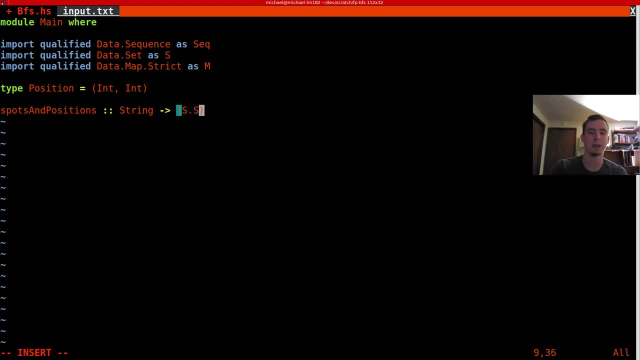 So it's going to take in the text of our board And it's going to return back a set of position as well as a map from a number. So one of our numbers here in this case, 0 to 4, to position. 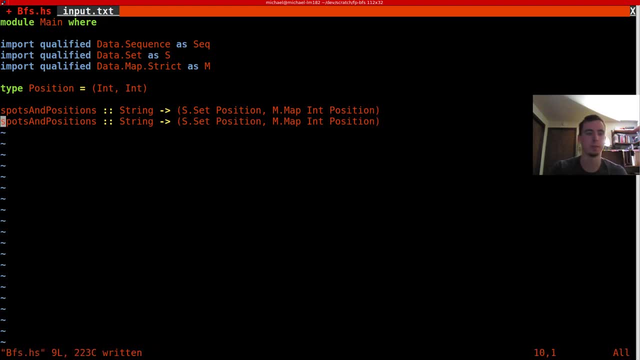 So where does that number exist in the board? So this is going to take in some text And then all we're going to do here Is we're going to do a fold And we're going to accumulate values as we go, Starting with an empty set. 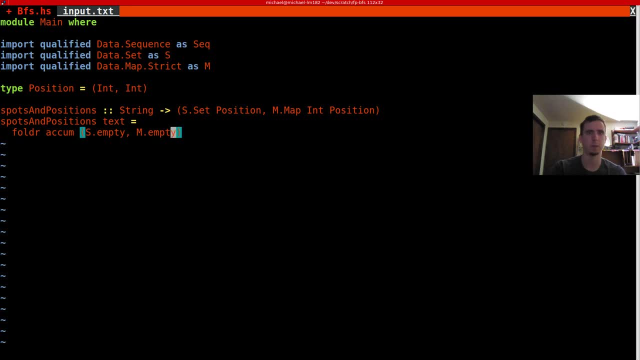 And an empty map And we're going to fold over the list of pairs and values. So position value pairs specifically. So first we can extract. We're using do notation here To loop over these values, So we're going to zip from 0 all the way up lines of text. 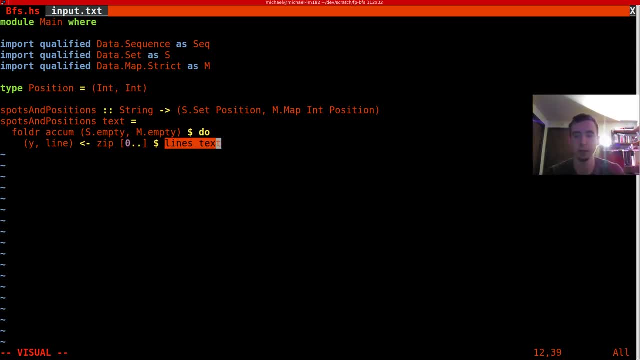 So, breaking this apart, First we're going to convert the text into a list of lines And then we're going to zip those lines with the indexes of the positions, And really starting at 0 here is totally arbitrary. The solution will work no matter what you put as the first index here. 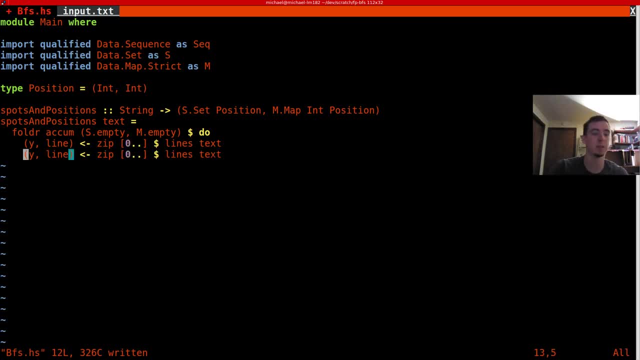 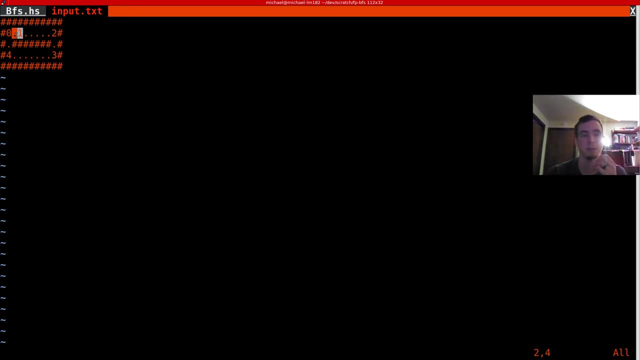 You can put totally anything you like. It could still work. It doesn't really matter. It's all kind of relative. If this was 50, 50. Then this would be 51, 50. It's still one away. 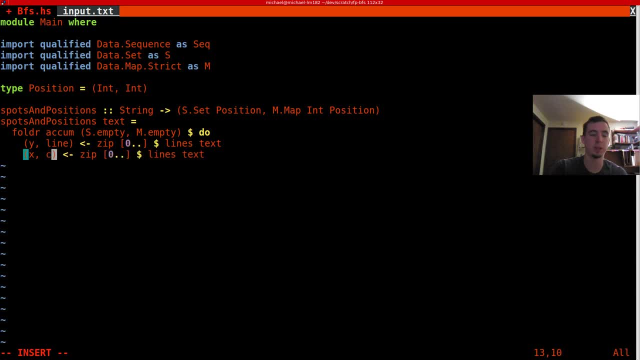 So we're going to do the same thing for x values, Except at this point we have a cell value And we're going to zip line. And again, it doesn't actually matter how we index these. Basically this, if you look back to the last video I made, 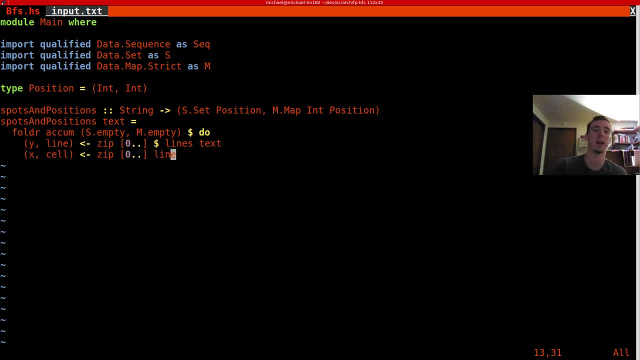 This looks a lot like the nested four reaches. It's very similar, It's kind of the same concept really. And then here we're going to actually return back our values And again this is going to be a pair of the position, So the xy pairing and the cell. 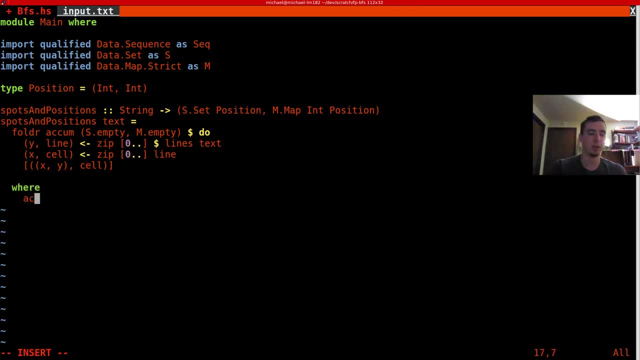 So now we have to define the accumulator So we can say where accum. And here we do a couple of things: If we're accumulating and we get some point and we get a dot, Well, we're also going to get spots and positions. 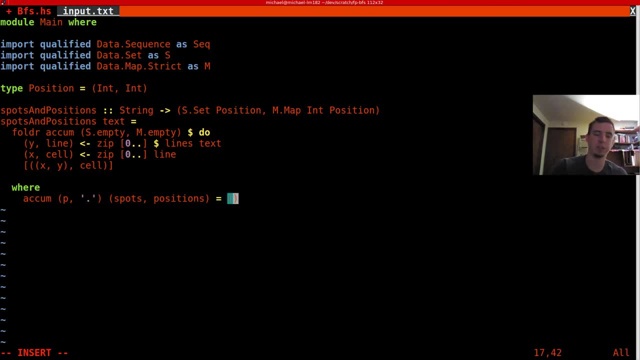 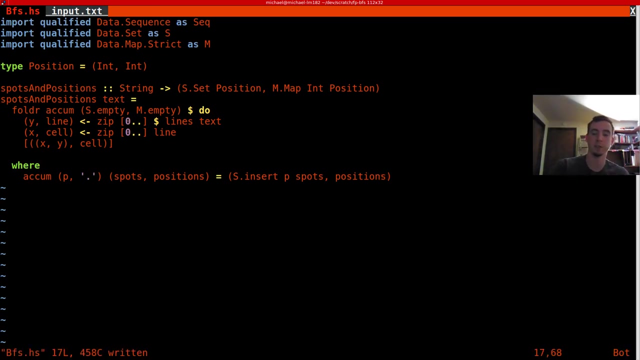 And what we're going to do is we're just going to insert that current position or that current spot into the spots And we're not going to change positions, because this isn't a number. So again, positions is a map from a number to its actual location. 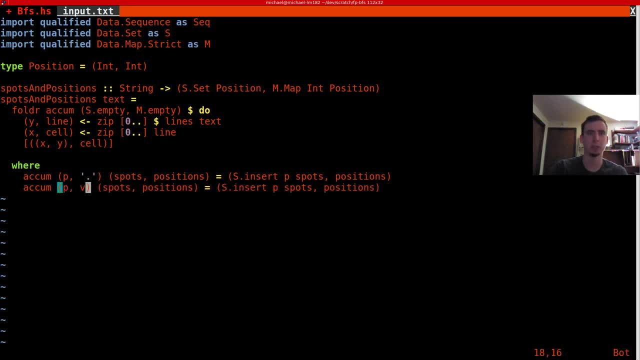 So if we get anything else, we're going to have to be a little more clever, And I'm actually going to use an alias here on this type Which will just let me reference it in a moment, using r to reference this whole thing, And I'm going to say if the value that we're looking at is an element of numbers. 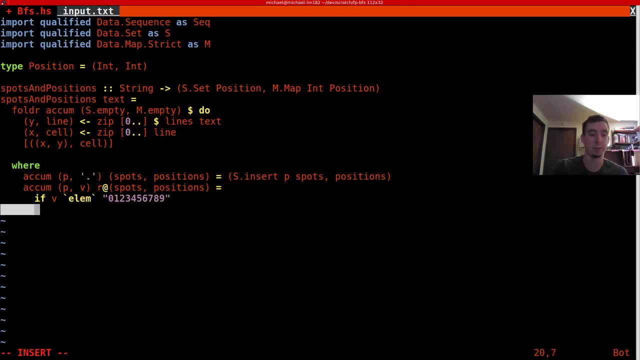 In this problem they only go 0 to 9.. Then we want to do something else. We want to return back r, So if the value is a number, Then what we want to do is we want to insert the position into the spots again. 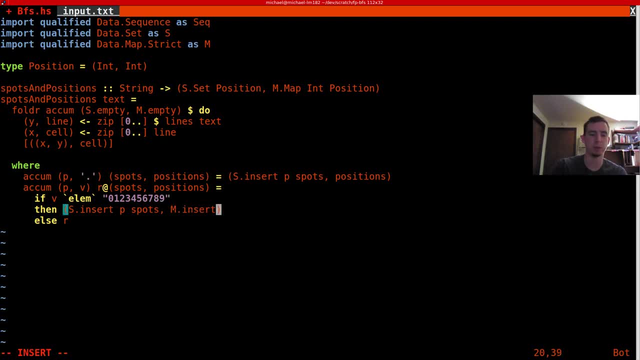 And then what we want to do is we want to minsert into positions the key of reading the value. Now, this might be a little bit confusing And technically this is safe by convention. You can tell it's safe because this element check will make sure that it can read as an int. 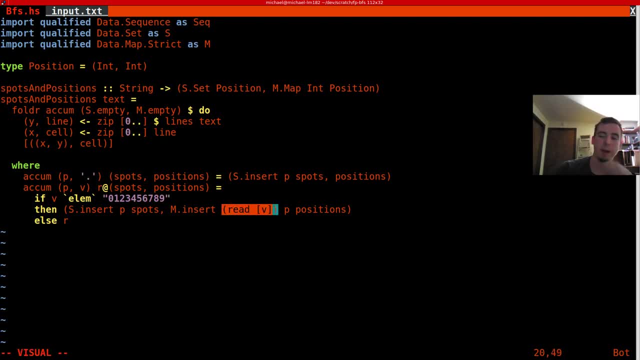 But if you just saw this code floating around, it wouldn't necessarily be safe, Because you can't necessarily always read a value from a string. You can't necessarily always read a number or an int from a string. But what I'm going to show you is what's happening here. 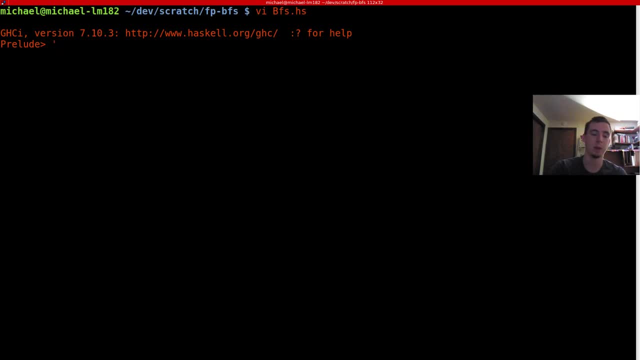 So if you had a character, let's say 5.. To make it into a string in Haskell, strings are just lists of characters. We can just put list around that. So that's what we're doing there And then read will parse it to something else. 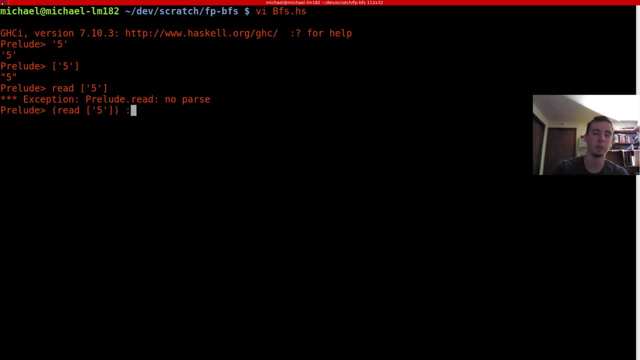 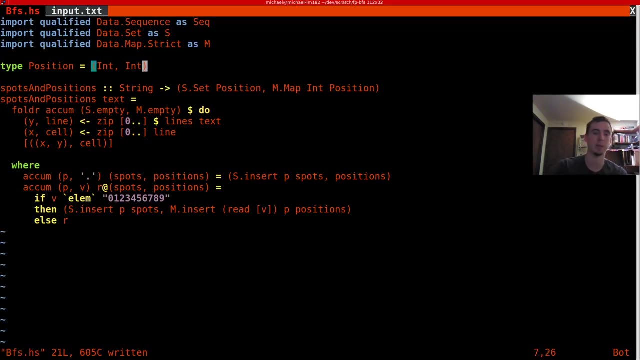 But the problem is, read has no idea what to parse it to here. So we're going to say, hey, read us an int. Of course, in my actual code here, since we're talking about ints via positions, Haskell can just kind of go and infer all of that for us. 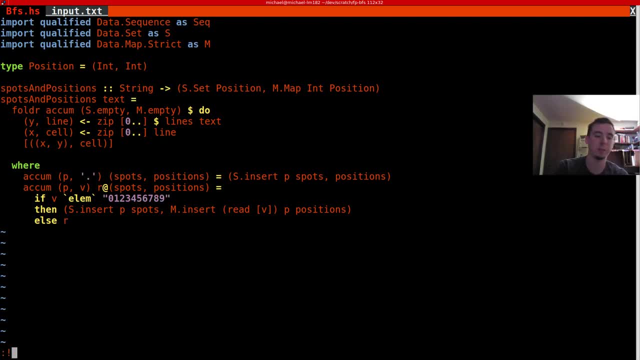 So this is what it takes to actually parse. Let me, as I'm going, let me just run this to make sure I haven't done anything silly, And I haven't. it's just complaining that main doesn't exist, which is okay, because we haven't written it yet. 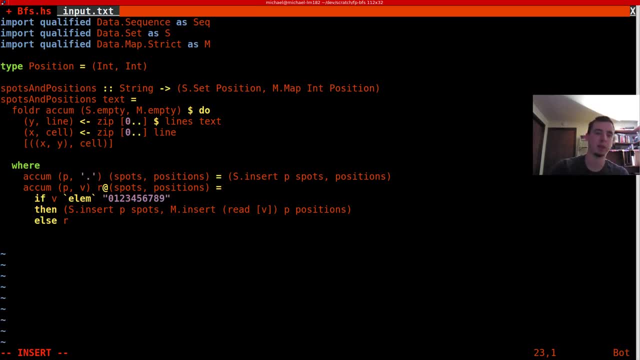 So the next thing we went on to write in the Python version is: we went on to write around, Which around basically took a set of positions, and in the Python version we didn't actually inject this, We just referenced it in scope. In this case, we're going to pass it down to the function because you'll see, it plays out a little more nicely. 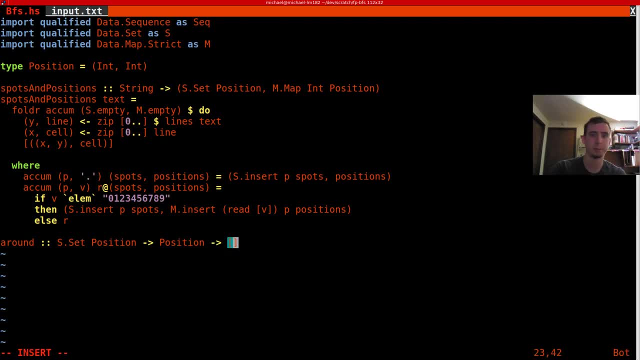 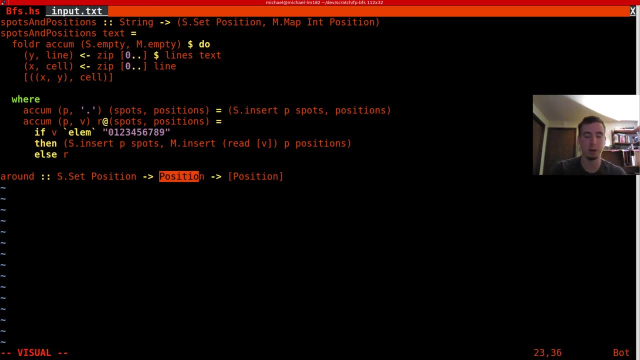 And then we're going to take back a position also, And we're just going to return back all of the positions that are valid around that position. So if this was a cell in the middle, its neighbors, if they were all dots or numbers, would all be valid around it. 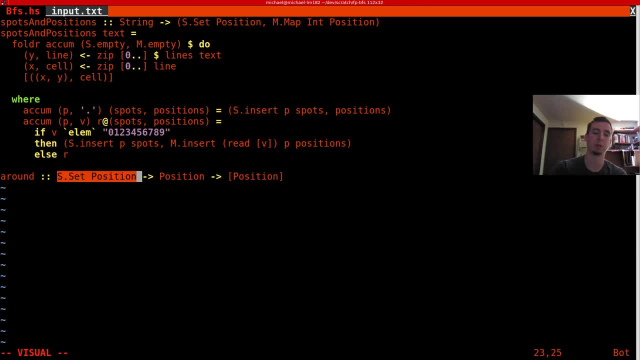 This is going to tell us what's actually valid, What's not- a hash character that we're not allowed to visit And, as you'll see in a moment, it'll tell us a little bit more too. So this is around and we're going to take in what's actually valid. 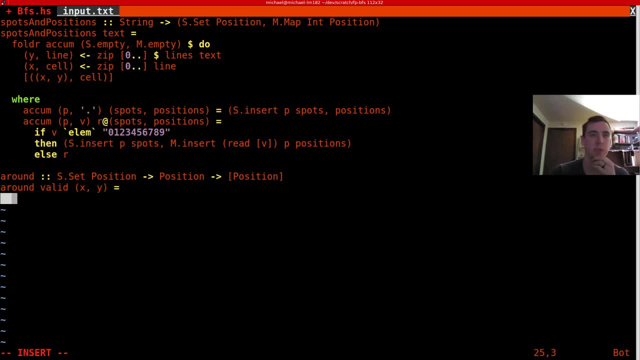 And we're going to take in our actual point, which we're just destructuring right there. So then, what we're going to do is we're going to filter smember valid And actually, when you call member, you need to put the value first. 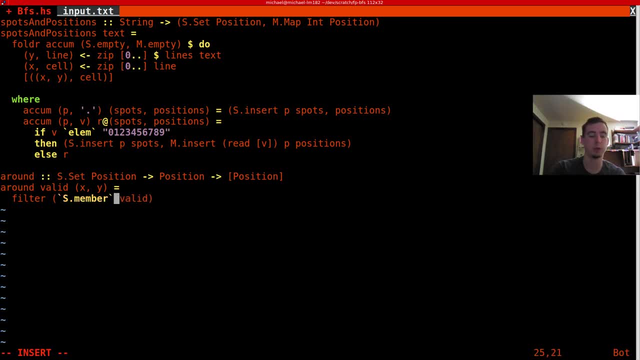 Which means this isn't going to work. now In Haskell you can use backticks to effectively flip the function, So that'll let us put the set as the first argument. And here we're going to do the same thing we did before. We're just going to say: this is x plus 1 y. 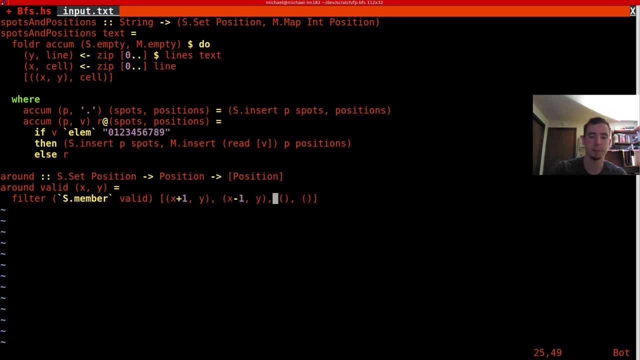 x minus 1, y, x- y plus 1.. And then x- y minus 1.. So this came out really nice in my opinion. So we're going to filter The list of things that could potentially be around, The ones that are actually valid to be around. 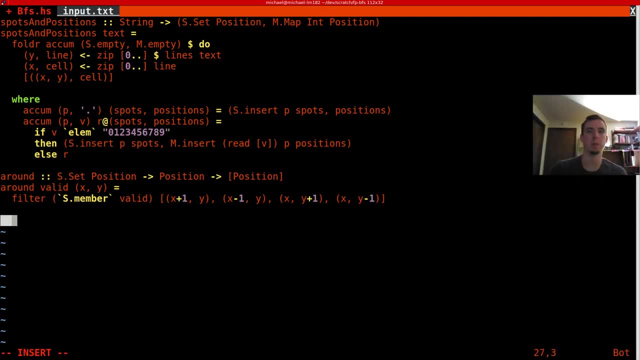 So that's kind of cool, Not too bad, And that's about it until we get to the actual breadth first search algorithm. So here we go. So dist is going to be our breadth first search algorithm And it's going to return the distance between two points. 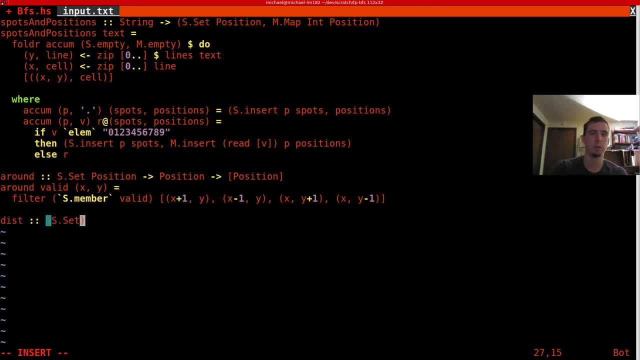 So it's going to take in our earlier determined set of positions To m map of int position. So it's going to take back, It's going to return, It's going to take in our spots and our positions And then it's going to take in some point that we're starting at. 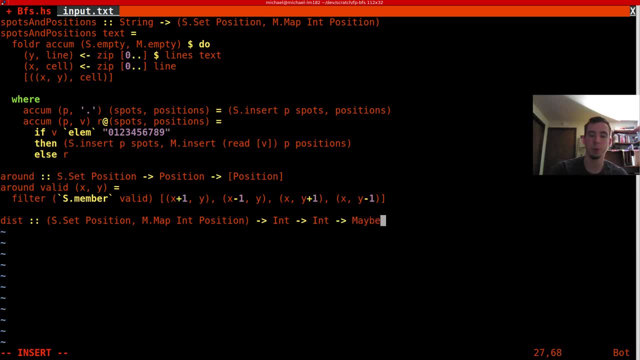 And then it's going to take in some point that we want to end at. And one thing we're going to do differently than the Python version Is we're going to return back a maybe int, And this is a little bit better, This is a little more safe. 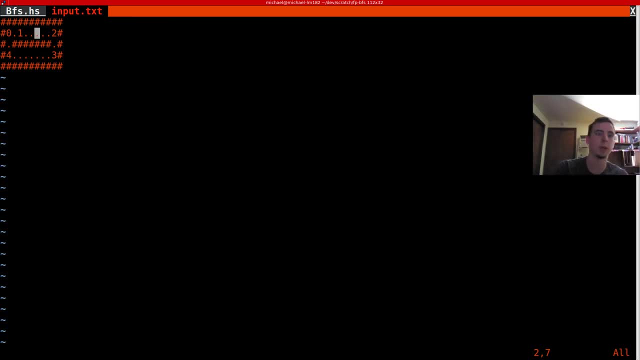 Because in reality, If we were given just any old input, We could have something like this: Where this is a hash and this is a hash, And then there's no way to get, Say, from zero to three. That's perfectly valid as far as input is concerned. 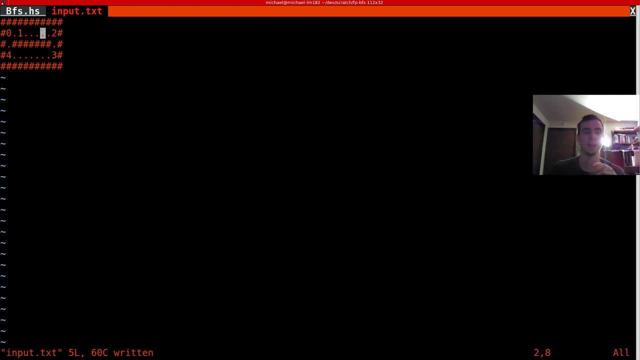 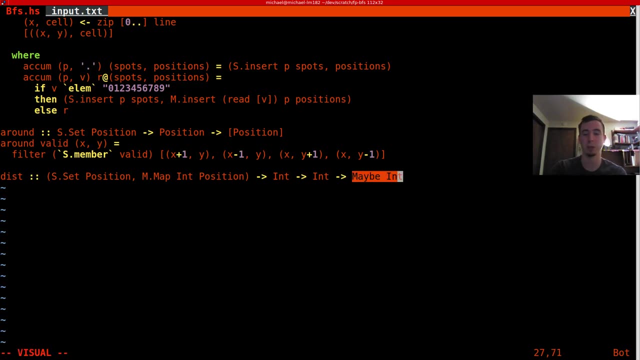 In advent of code, Unless otherwise stated, They tend to give you valid inputs, But in reality that might not happen, So we have to account for it with maybe, Which is really just another way here to say No path exists. We weren't able to find a path from, say, zero to three. 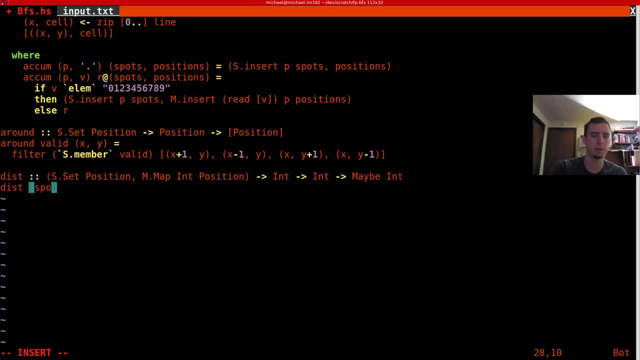 So dist is going to take in, As I said, spots and positions, And then it's going to take in some source And it's going to take in some dest, And now we're going to use do again here, Do syntax. And the nice thing about do syntax: 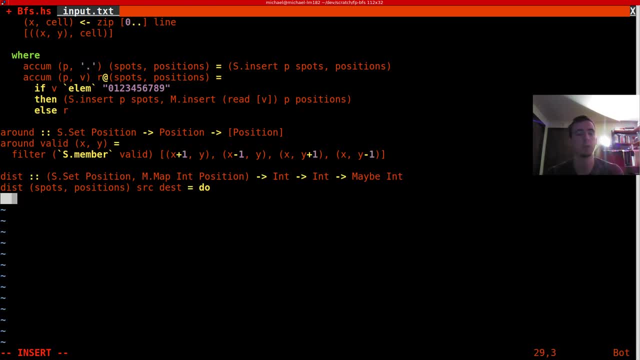 Is that it works on any monad in Haskell, So we used it for lists earlier And now I'm going to use it for maybe. So to get the actual source, We're going to do an mlookup, A map, lookup Of source and positions. 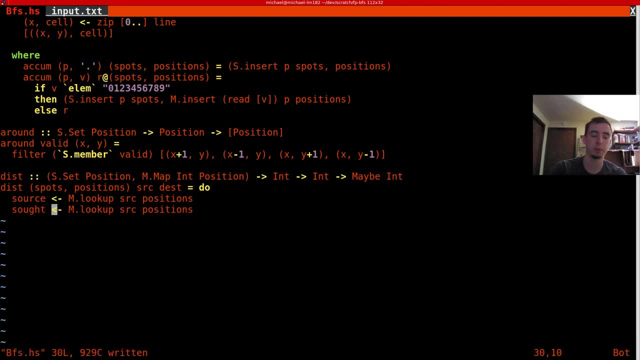 And then to get the actual destination, Which I'm going to rename as sought. So source and sought are what we're seeking after We look up the dest in positions, And then what we're going to do Is we're just going to delegate to a helper function. 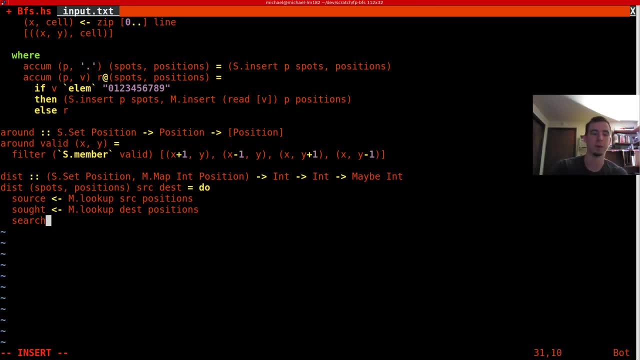 Which is going to be called actual search. Do the search for me, And that's going to have to take in the sought value. And also we're going to pass two things, Exactly like we did in the Python version. We're going to pass what we've already visited. 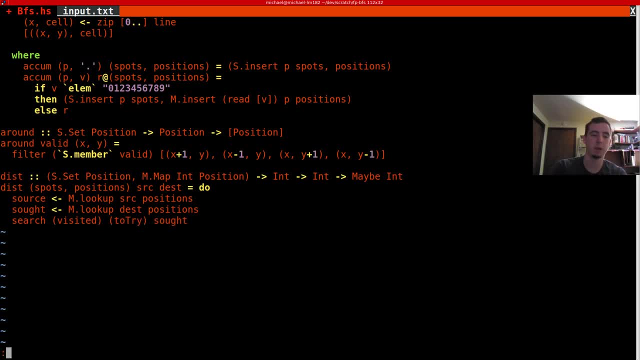 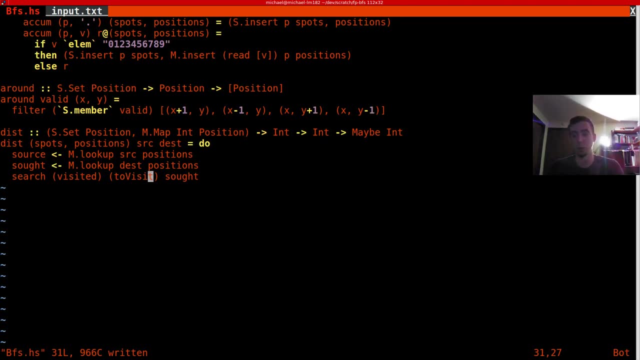 And we're also going to pass what we have to try- Or maybe to visit is a better word, So we're going to pass what we've already seen. We shouldn't look where we've already looked. It's a waste of time. 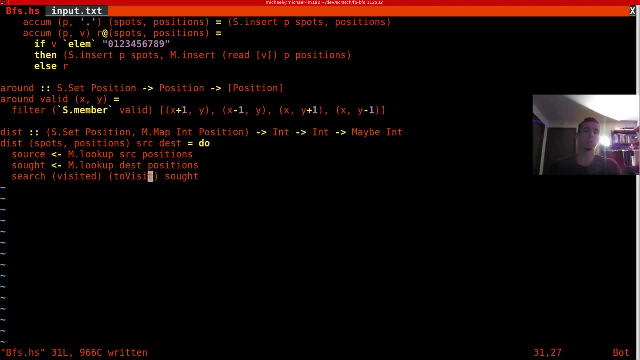 And we'll end in infinite recursion. And we also have to pass what else. we have to check Around where we've already checked. So visited is going to start as a set Singleton. So a singleton function just builds the value that it's constructing. 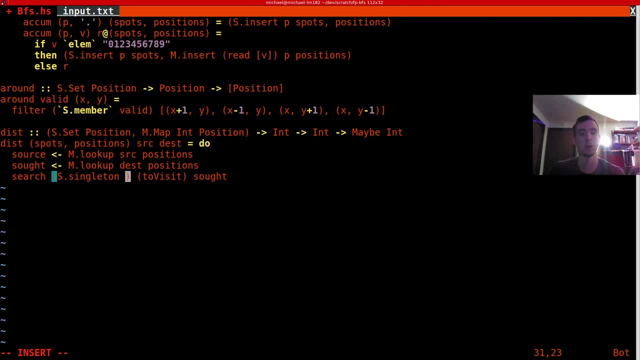 With one element in it. So this will build a set with one element, And that element is source. So we've already visited source. Because we're going to build a set, We're going to build a seeksingleton of the source and zero as a pair. 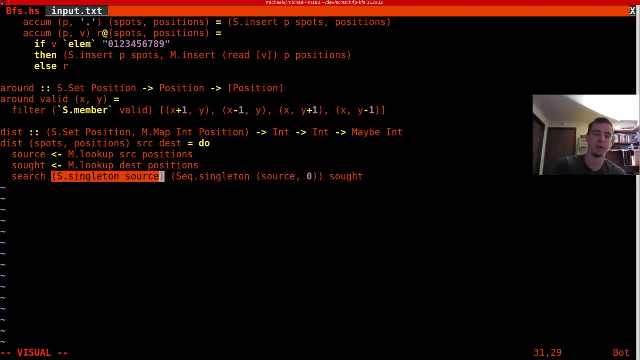 So search, if you look at its type, it's going to take in a set of what we've already seen And then a sequence of things that we still have to try. So positions: we haven't yet really investigated, or investigated their neighbors. 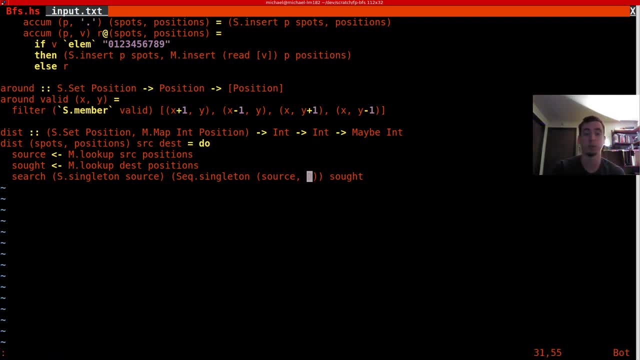 And how far away they are from source. So source is zero from source. What does our actual search look like? Well, our actual search, as I said, it's going to take in what we've already visited. It's going to take in to try or to visit. 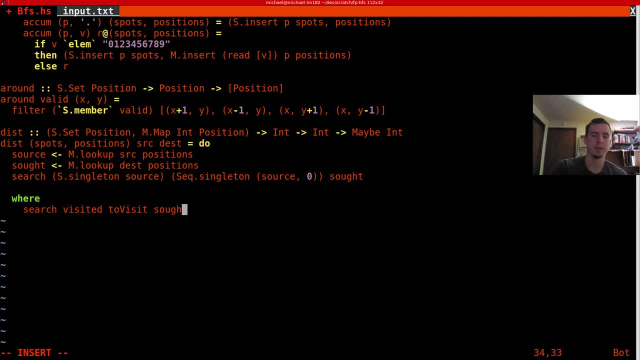 I'll call this to visit. That's probably a better name, And then it's going to take in the sought value. Now I wish in Haskell there was a way to just reuse this name down here in this, where scope, You can reuse names up here. 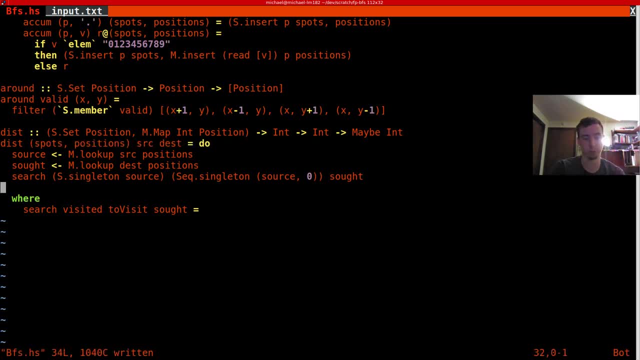 But you can't reuse ones that are bound in due notation. There might be an extension for that. The Haskell answer you tend to see is there's an extension for that, But that's neither here nor there. So what we're going to do is we're going to use case seekviewL to visit of. 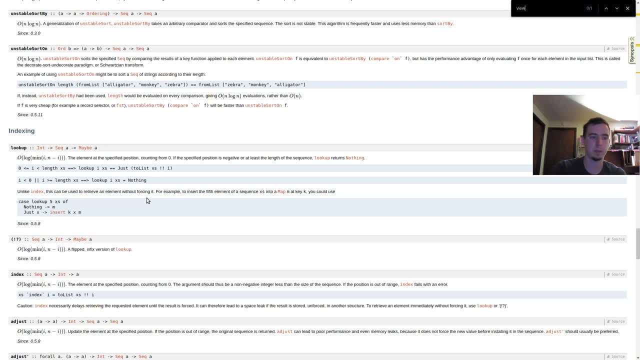 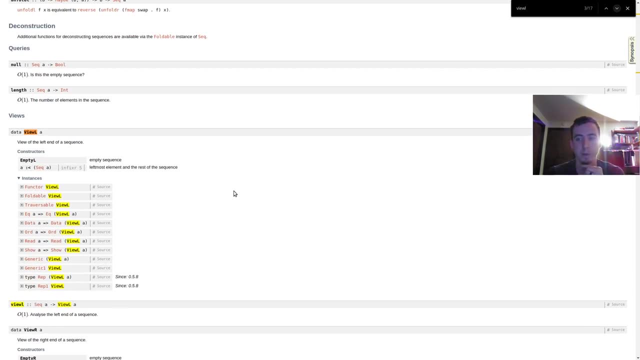 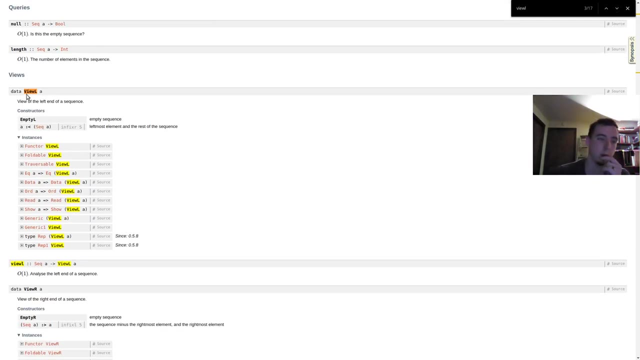 So what viewL does? I'm going to pull it up right now. ViewL is a way to essentially take the first value of our queue. Our queue is first in, first out, basically. So What we're going to do is viewL will return back either an empty L or the head of the list. 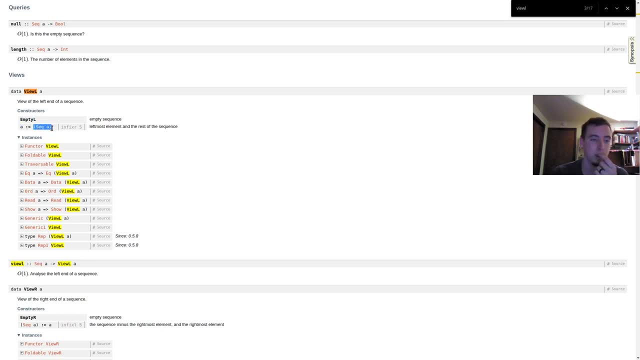 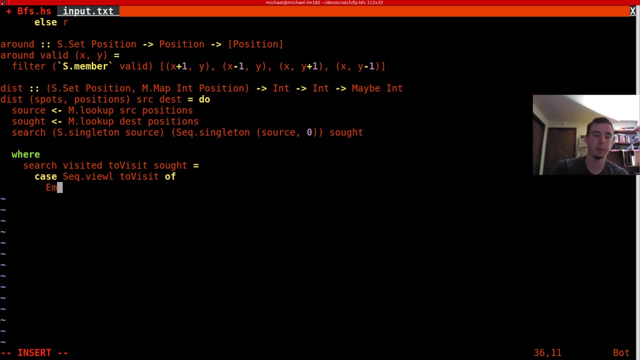 the first element of the queue, the one we have to pull, and the rest of the elements. So the cases then actually look like empty L And if we get an empty left, well, basically that means we found no elements, We have nothing left to try. 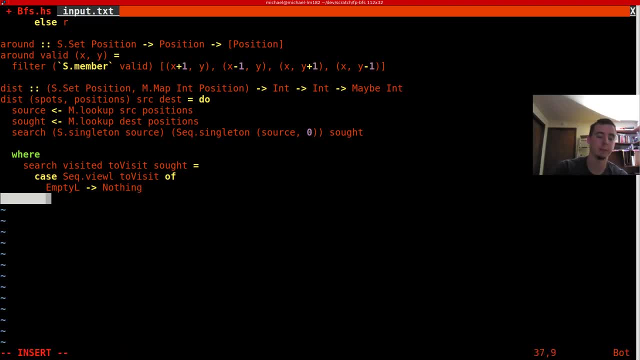 We've exhausted all of our possibilities. This is a nothing. And we have to say seekviewL. And we have to say seek because we namespaced everything as seek. So next we have to go and we have to actually say what the value is. 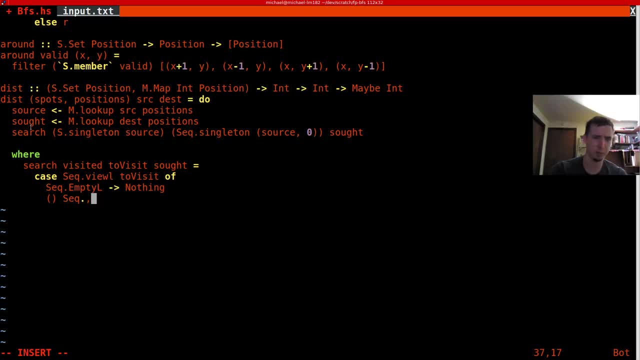 So this is seek, whatever this little symbol is, which is kind of cool looking: Colon arrow, Rest- Yeah, That's what we want, And then this is going to be: basically, we can destructure this right here, which is another sweet thing about Haskell pattern matching. 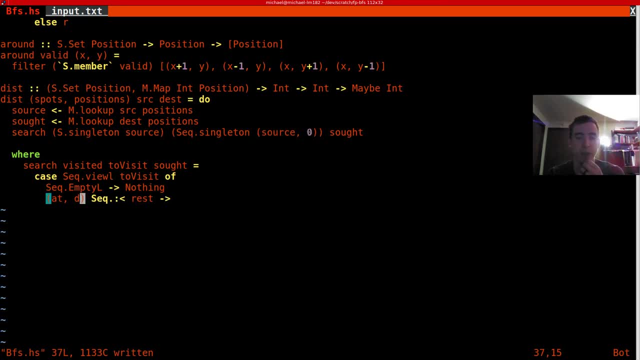 So here we're just pulling out the thing we're currently trying, And it's current distance, basically. So, basically, what we want to say is, if we're at what we're seeking, So if we're at the sought value, then we found it in the distances where we are. 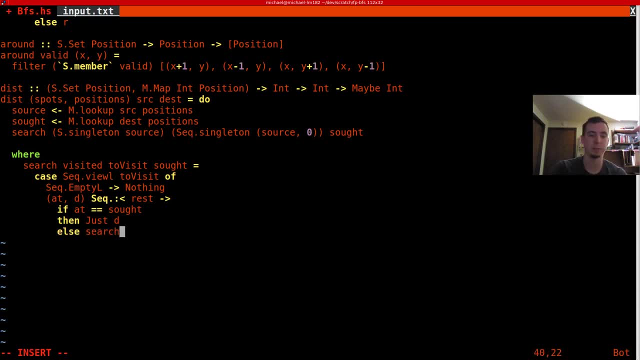 Otherwise, what we want to do is we want to search again, But we want to track some new visited values. So I'll say visited prime And we also want to say the rest of the values, which is? this value up here Should be appended to or concatenated with is probably a better way to say it. 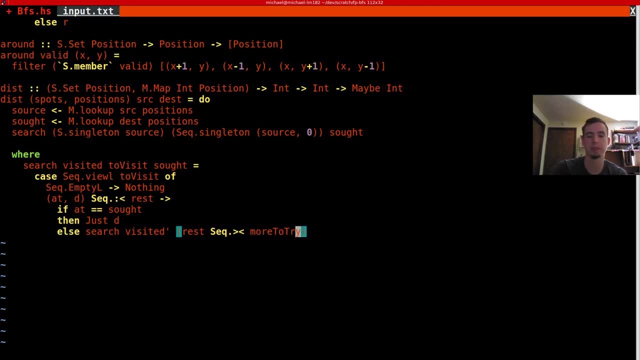 Some more that we have to try More to try More to visit later And of course we have to recurse and pass sought down. So let's go ahead and build up these couple of missing values. So we'll use let here. 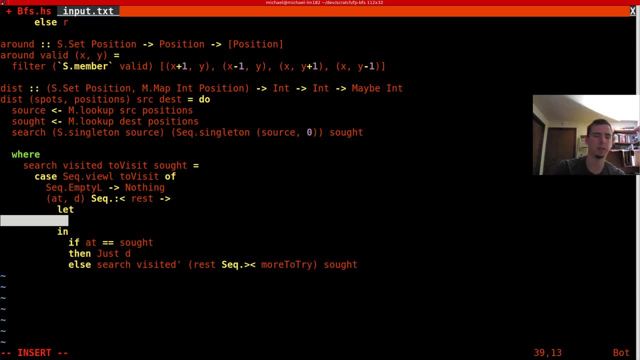 So we can say let in. So basically, first let's get the neighbors. So the neighbors are going to be around where we're currently at- And this is kind of the cool part- You almost want to just say spots here. But what we can do is we can use set difference to say we want the things that are around us, that are spots that have not already been visited. 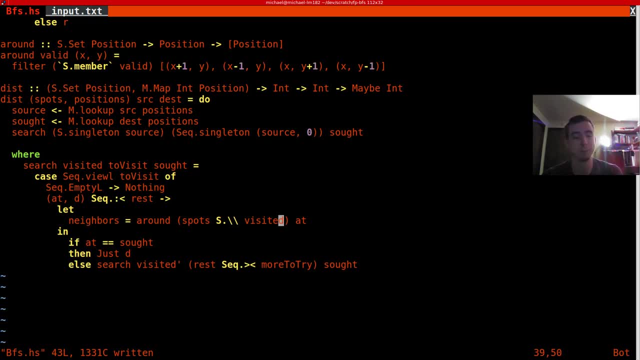 So basically, this is going to get the neighbors that we haven't seen already Super cool, And then we have to adjust our visited, We have to add new things to it, And that's going to be the union Of visited and set from list of neighbors. 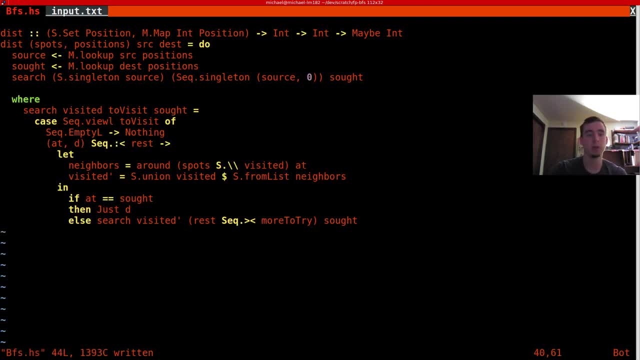 So we have to add all of the neighbors that we're going to look at now to the list of things that we've already visited. So, and then in the end, we have to say more to try. So what else do we have to try in addition to rest here? 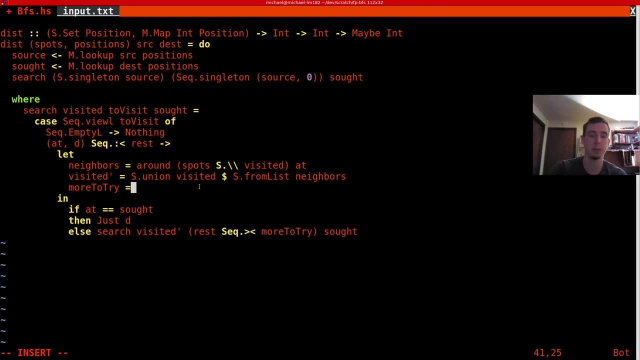 Just to keep our queue in the right way, Keep our queue in the right order. We're going to use seek, that from list, And this is going to basically take our neighbors, And what we're going to want to do is we're just going to want to map a neighbor and say neighbor, and then D plus 1.. 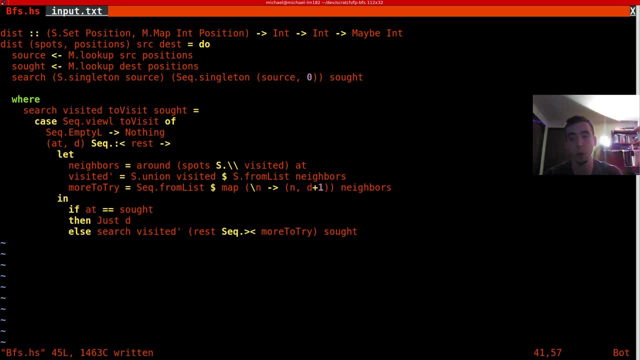 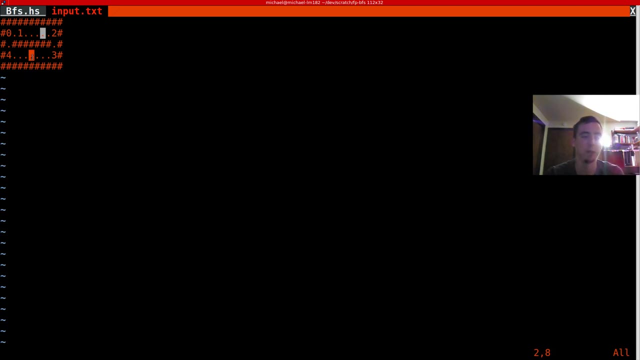 So the idea here is: all of our neighbors are one more away from the step that we just took. basically, So if we're at some position here, let's play an example. If we're at this position, however many steps we took to get here, this is one more away. for example, 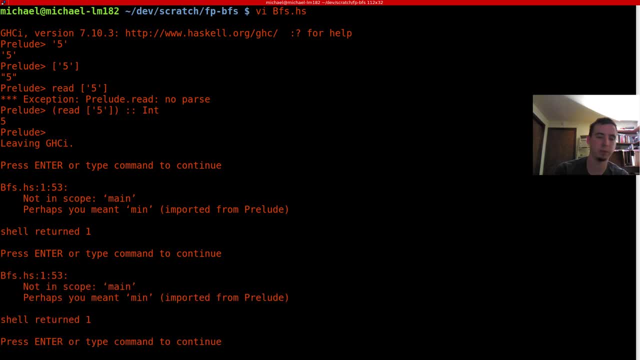 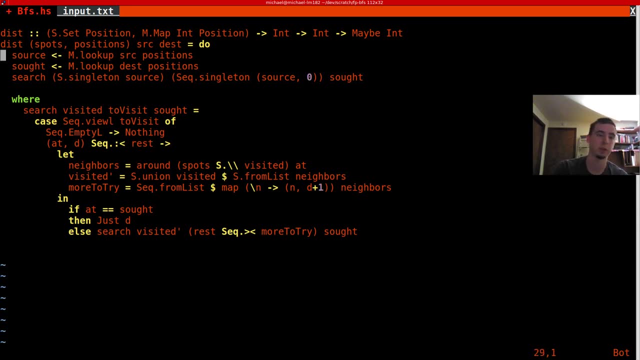 So I think that's actually it. Let me go ahead and just run this and make sure it's still failing for the same reason it is. So now we need to write a little bit more boilerplate, But basically that's it. This is our breadth-first search. 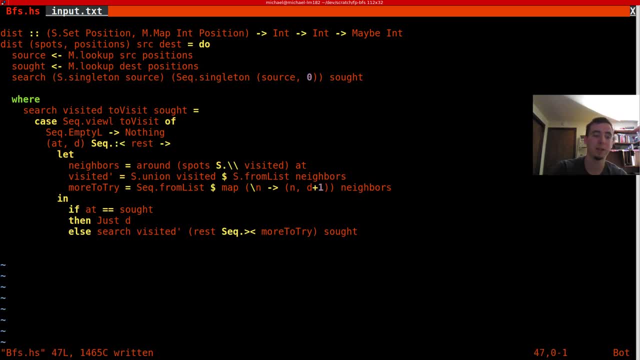 As in the Python example, we can modify it to become more robust. This version is safer because it doesn't just assume every path exists, as we'll see in a moment. So, basically, what we can do is we can read in the text of the file: 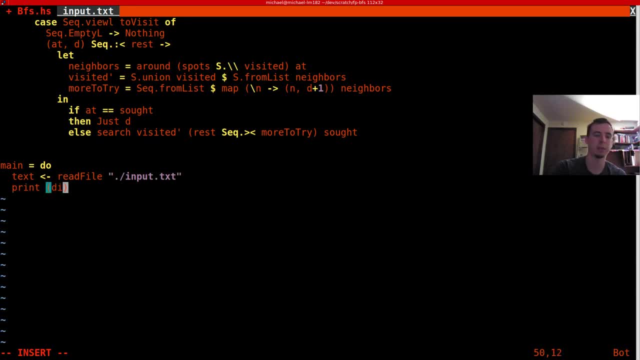 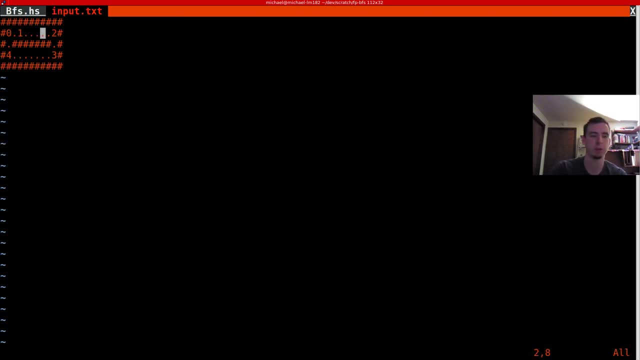 So we'll read in inputtext And then what we'll do is we'll just print out the distance of spots and positions of the text, And let's just try 0 to 3 first. So 0 to 3.. This one was 10, if I remember correctly. 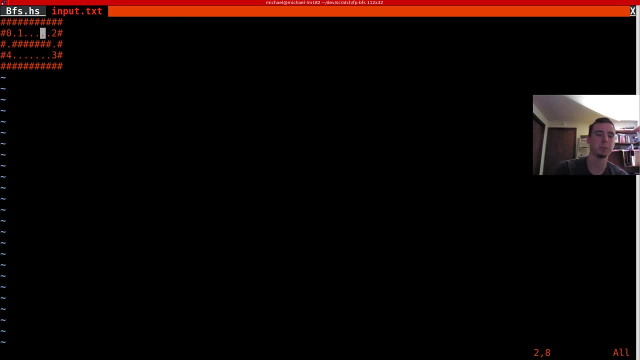 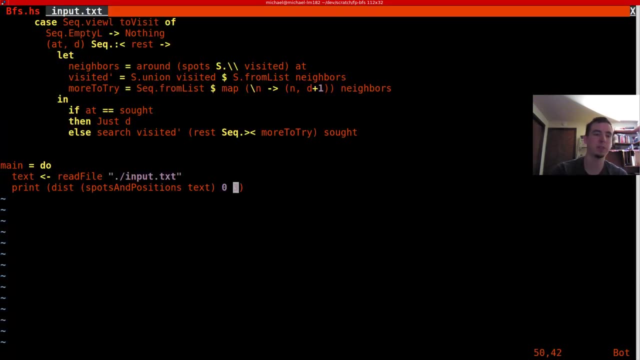 So if we run it, we get back just 10.. Wonderful. So now, just for fun, let's go ahead and let's block the path. There should be no way from 0 to 3 now. Oops, Block file. Yep. 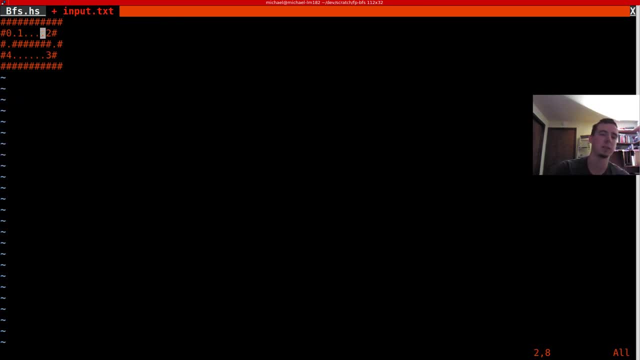 Nothing That's cool. Let's go ahead and let's try to make life a little different for the puzzle, for this problem. Let's just move. I don't know What's something fun we could do here. We could make a new. 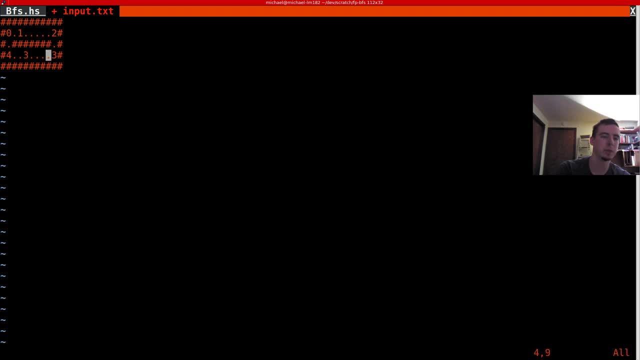 Let's put 3 here, so that it's not 10 away, And then let's see what that does. That should take the short path right around the corner here, So it should go 5, 1,, 2,, 3,, 4,, 5.. 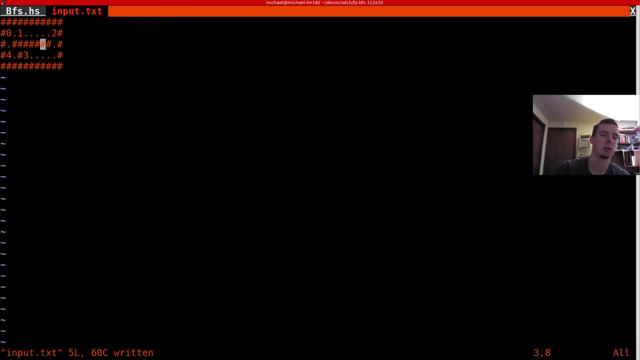 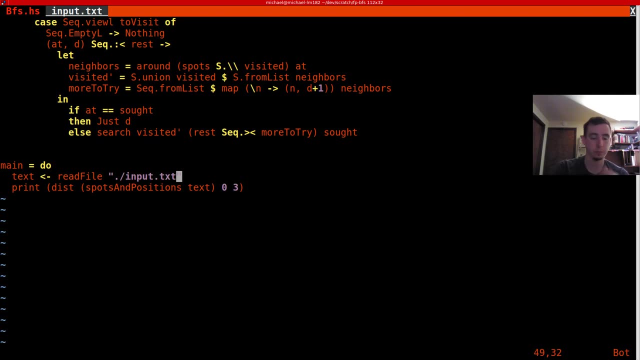 Yep, And then, if we do this, it should have to take a long path all the way around, roughly, I don't know- 15. Yep, 15. Awesome, Cool, So that's it. Hopefully this was useful to you. 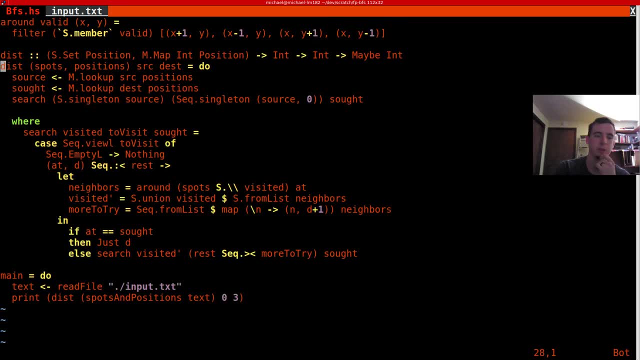 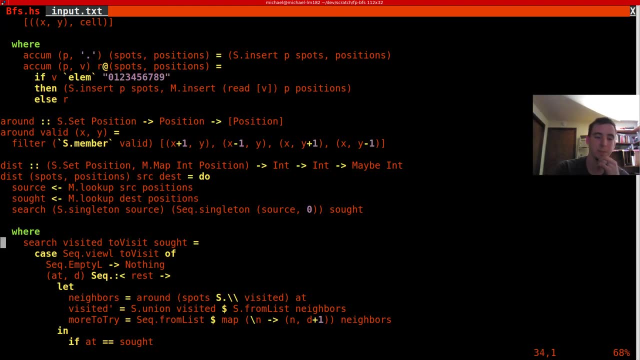 I think it's exceptionally kind of cool to do it in a functional style, And I think it. I really do think this problem lends itself well to a functional style. I think that seek is a nice way in Haskell to represent a queue And thanks for watching.